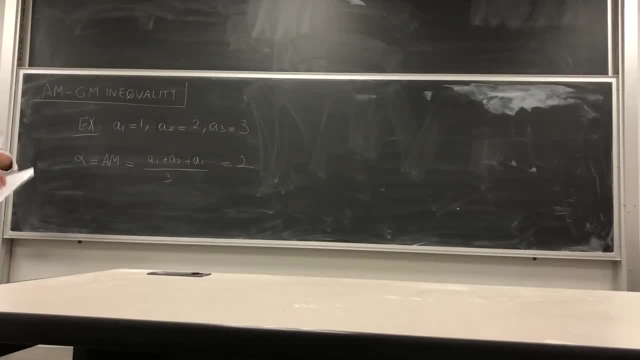 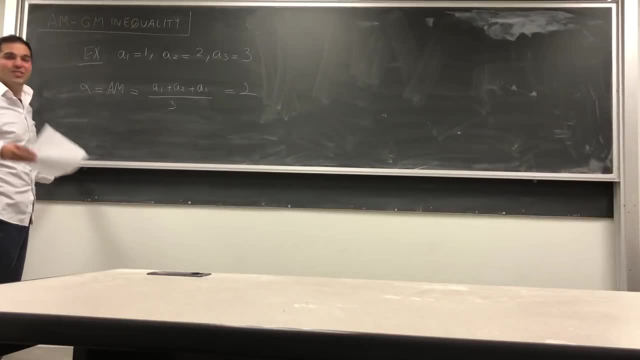 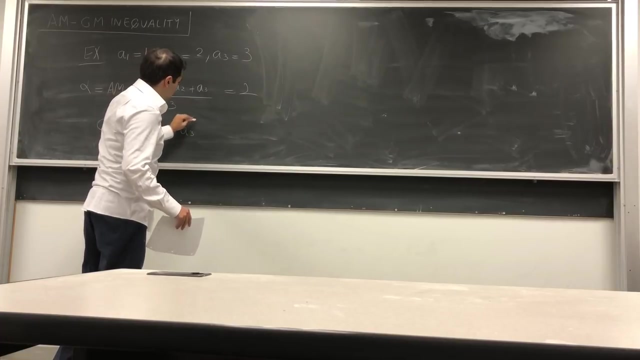 dividing it by the number of values Turns out. there's also another way of doing this: taking a mean- what do you mean? which is called the geometric mean, and all you do, instead of adding up the values, you multiply them. so a1 times a2 times a3, and then this: 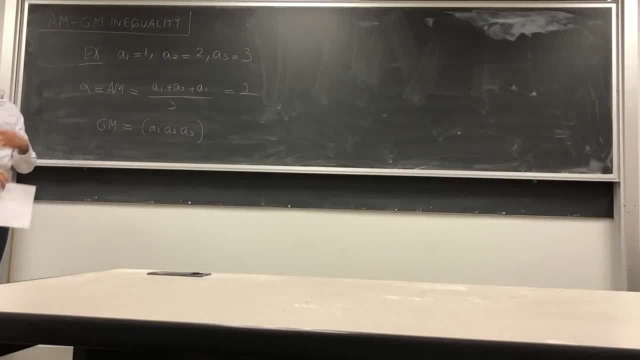 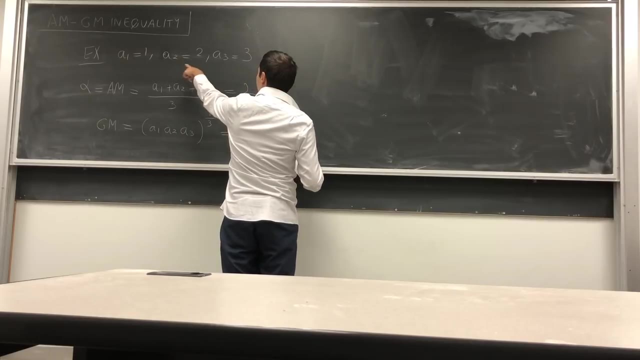 might get very big, but in order to have a number which makes more sense in this case, instead of dividing it by 3, you take the cube root of 3, so 1, over the number of values, and if you do that, you get 1 times 2 times 3, which is 6, and you: 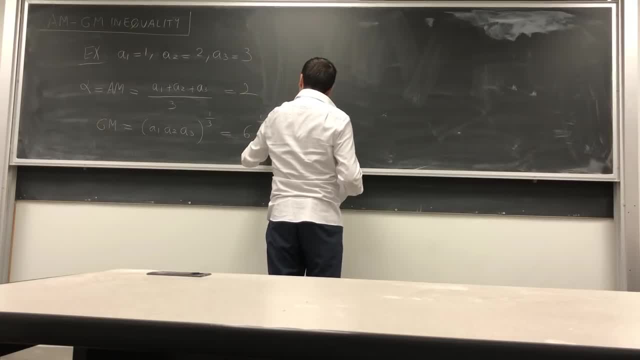 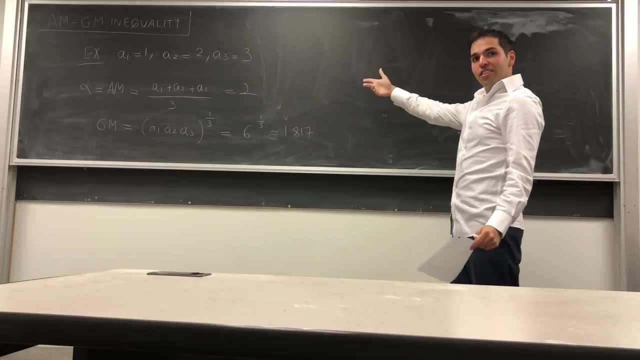 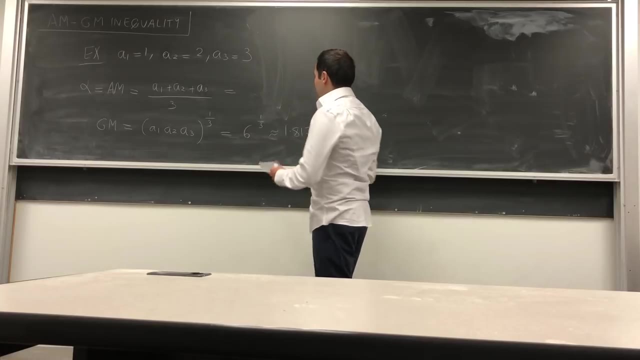 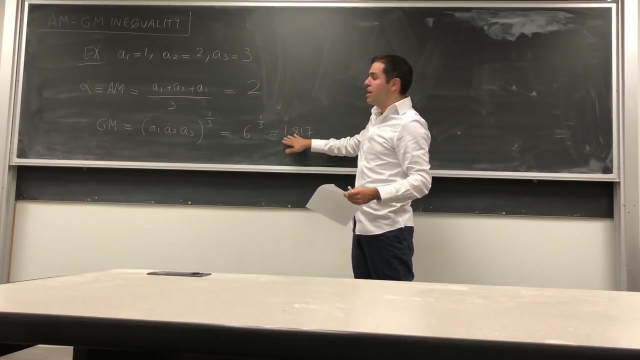 have the cube root and, if you like, this is roughly 1.817. and now notice. so those are two ways of taking the mean of something. if you compare those two numbers, 2 and 1.817, you notice that this number is bigger than this one. in other words, in this example the arithmetic mean is: 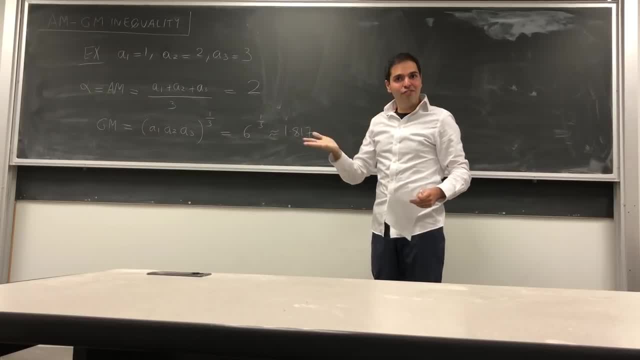 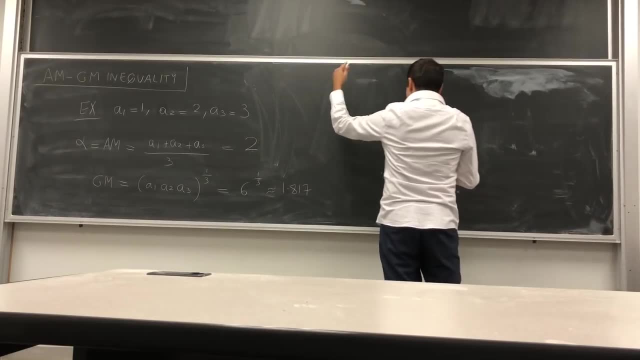 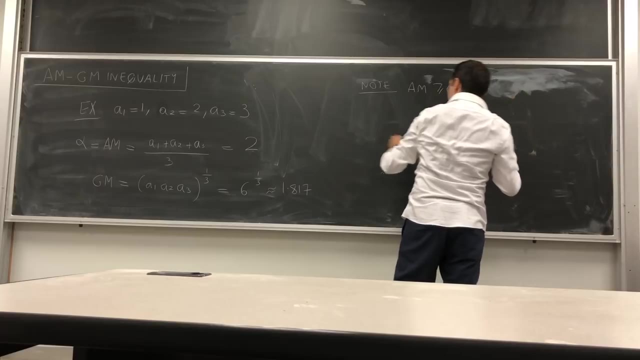 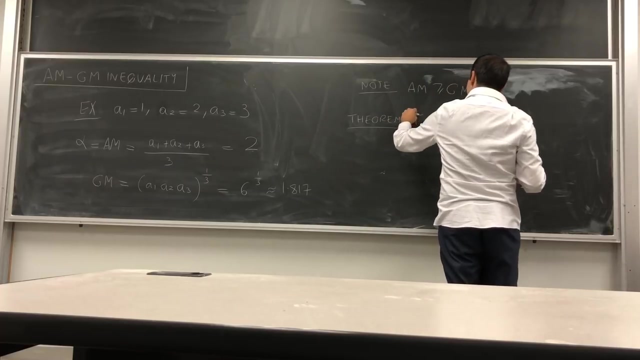 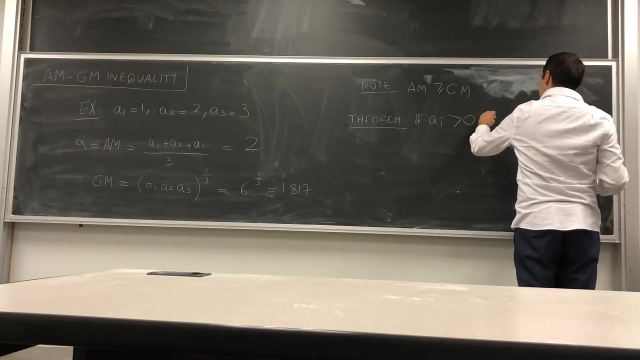 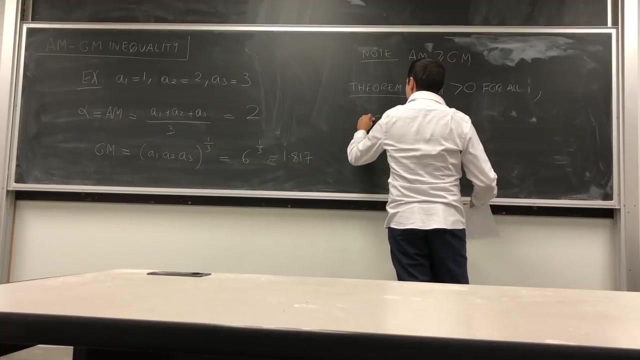 greater than the geometric mean and in fact turns out this is always true. the arithmetic geometric mean, inequality- a, n is greater or equal to g, m and the theorem is: if all those values are positive, if a, i is positive for all i, then if you take the arithmetic mean, so if you take a1 plus blah, blah, blah, plus a? n divided by n, 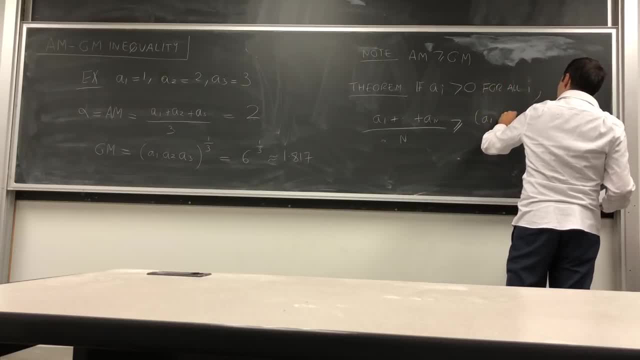 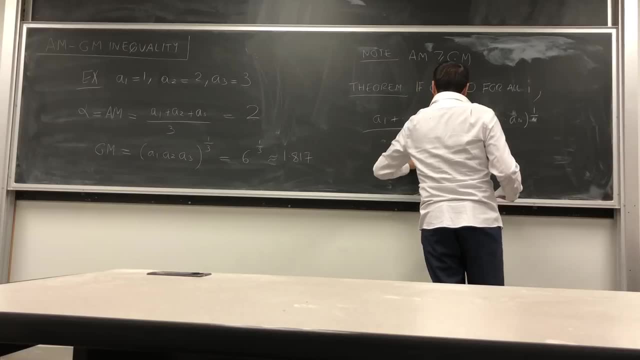 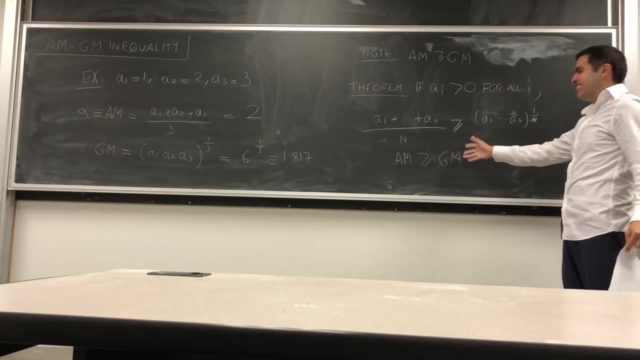 this is always greater or equal to the product a1 up to the n of the nth root of this. in other words, again, the arithmetic mean is greater or equal to the geometric mean. so good thing that your classes are not curved by the geometric mean, because the 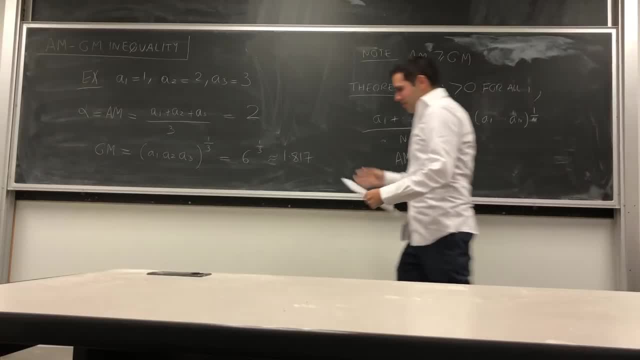 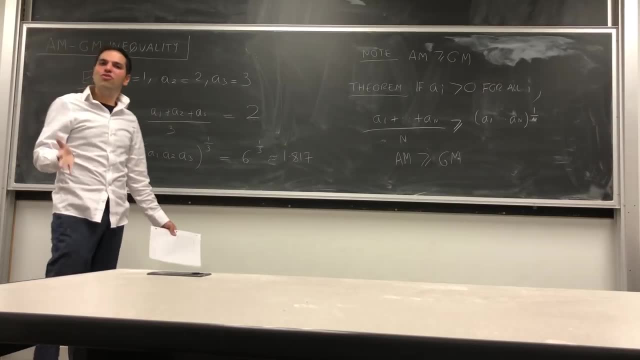 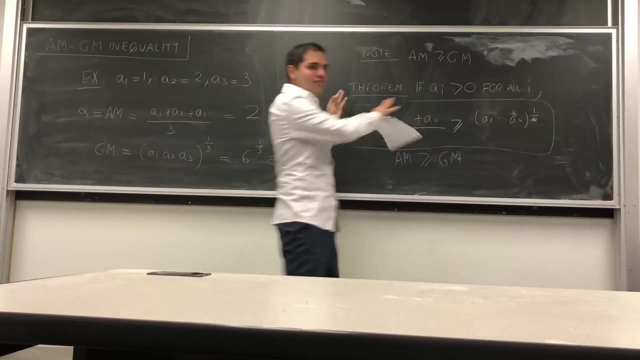 arithmetic mean is better, and of course you might say, okay, great, but it turns out this is one of the theorems where i think the proof is even more amazing than the theorem itself. so let me prove this, and again: proof due to alex zorba. okay, step one. 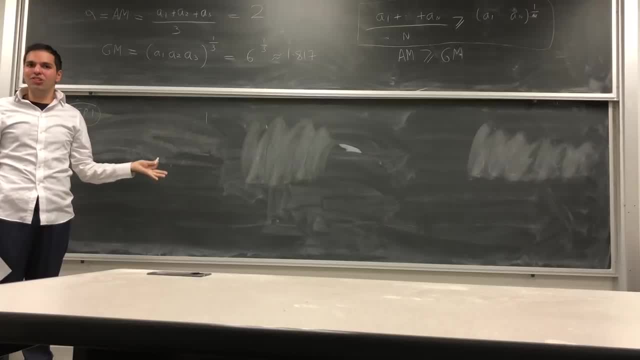 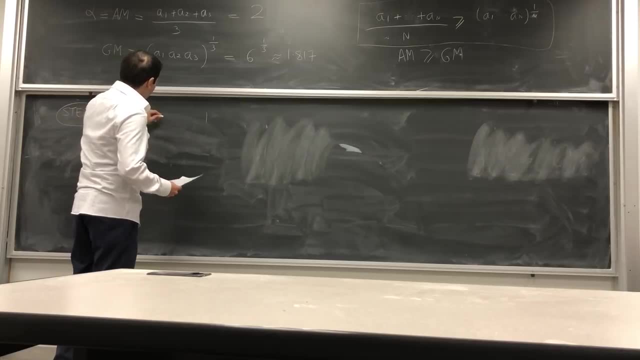 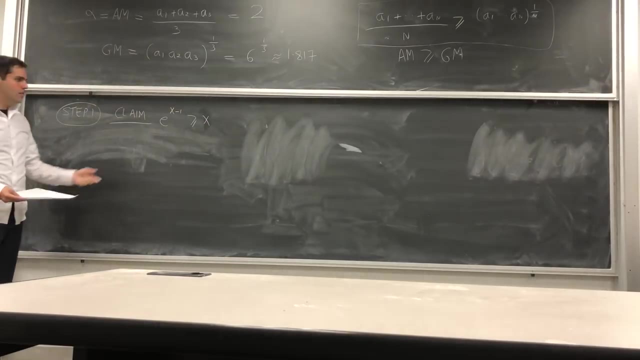 let's show something that at first sight has nothing to do with the a, m, g, m inequality. namely, let's show, or let's claim, that e to the x minus one is always greater or equal to x. so in other words, if you divide e to the x by the number e, it's always greater or equal to x. 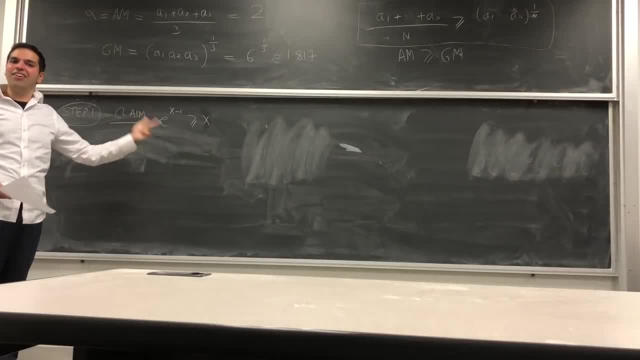 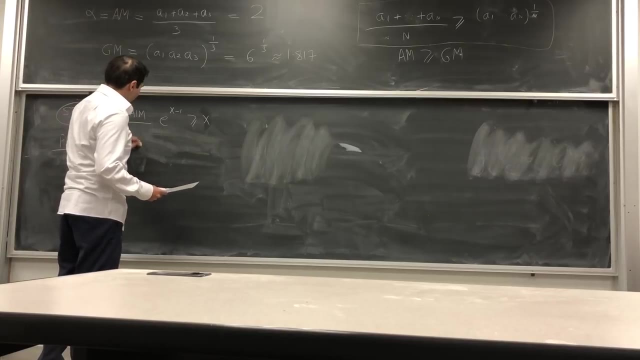 and this is a very typical, you know, calc one exercise, because in order to show a function is positive, or in order to show an inequality, let's consider the difference. so proof that f of x, the e to the x minus one, minus x, and let's hope that we can show that f of x is greater or equal to 0, and in general, 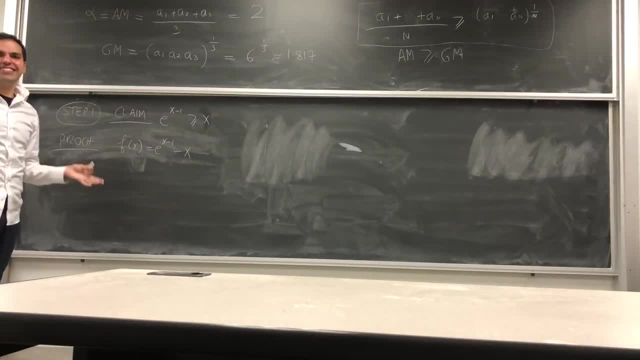 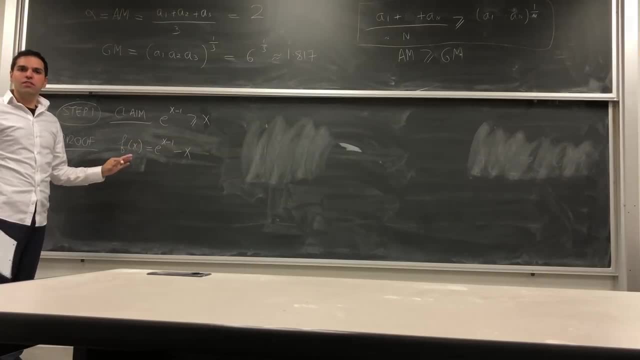 this thing doesn't work, but luckily in calculus classes this technique does work. So first of all, let's calculate the derivative and figure out where the derivative is 0. Because the idea is, you want to use some critical point argument and maybe show that the minimum 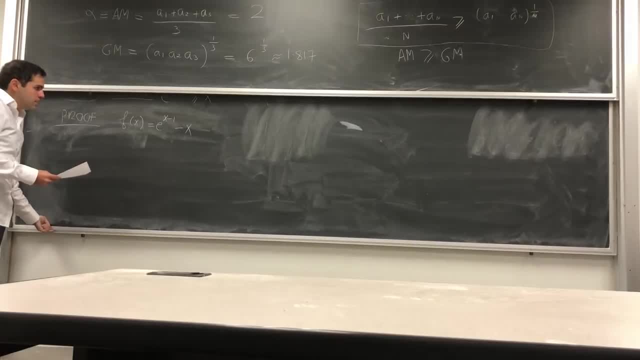 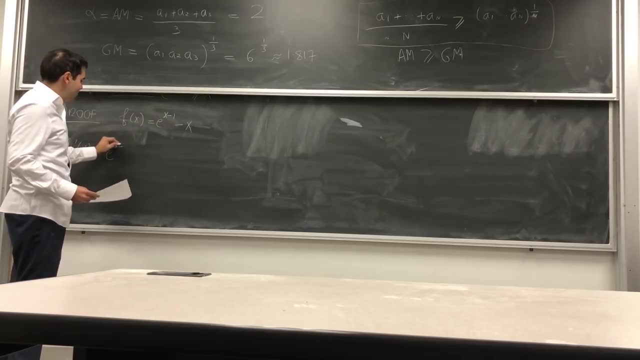 of f is 0.. So let's calculate f prime, f prime of x. well, derivative of e to the x minus 1 is still e to the x minus 1, and then the derivative of x equals to 1,. and let's now figure out. 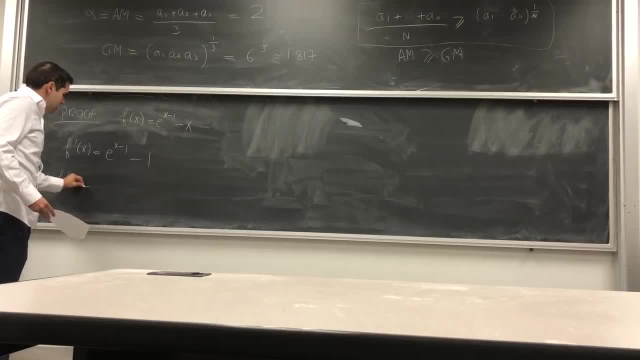 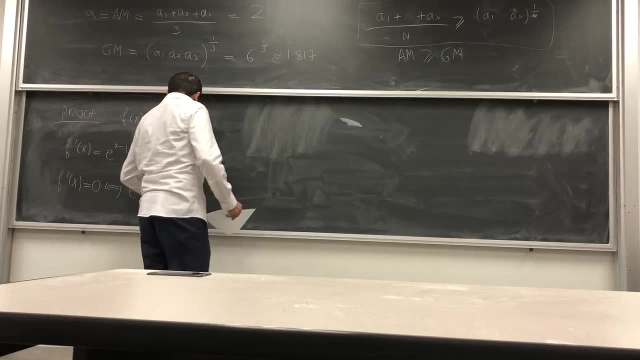 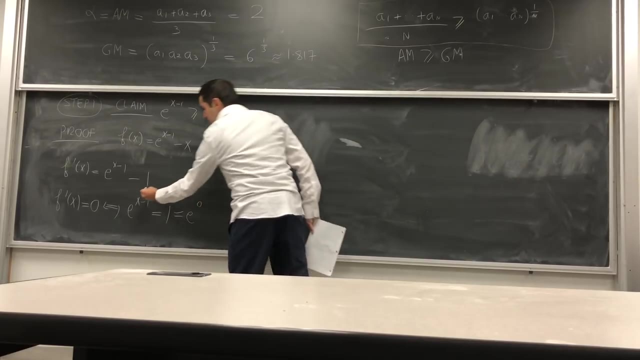 when this is 0.. So f prime of x equals to 0 if, and only if, e to the x minus 1 is greater or equal to 1, or remember, 1 is e to the 0, and so e to the something equals to e to the something. 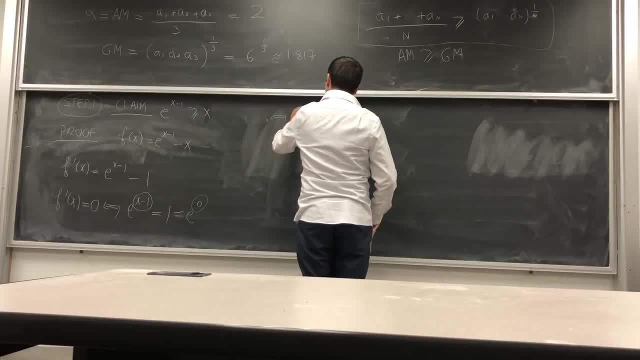 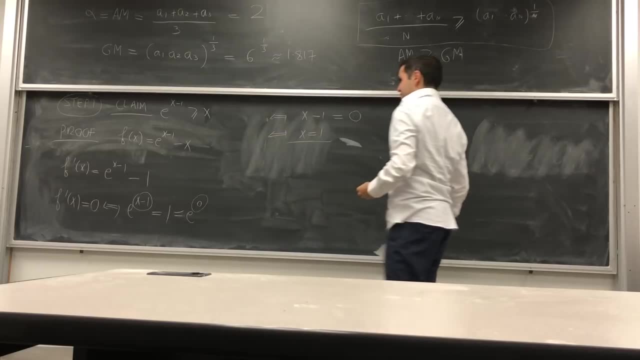 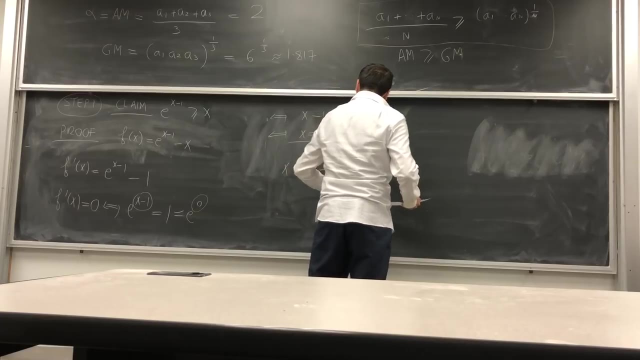 if, and only if, those two things are equal. So x minus 1 equals to 0, if, and only if, x equals to 1.. So if you want to draw this on a table, we get: if x goes to minus infinity, 1 and infinity. 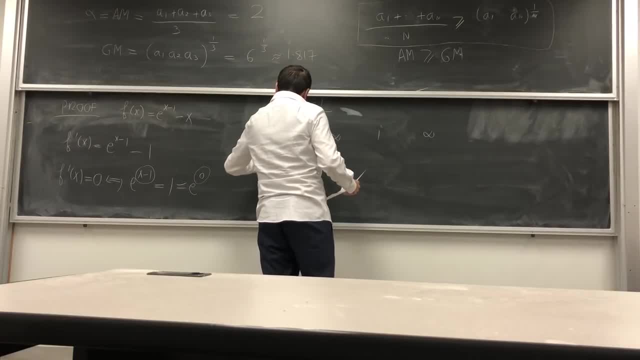 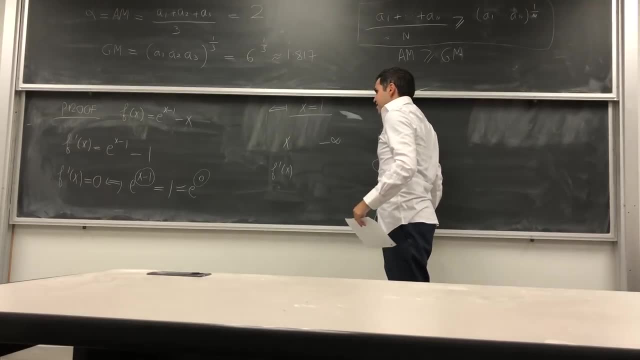 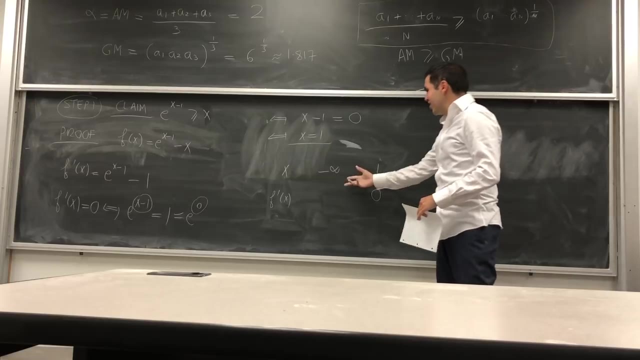 0. Then f prime at 1, it's 0, and also almost analog, not analog, you know- in an equivalent way. OK, it's easier to pronounce. you can show that on this interval minus 1 to minus. 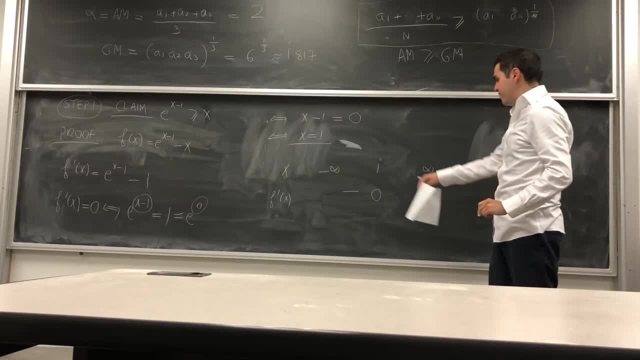 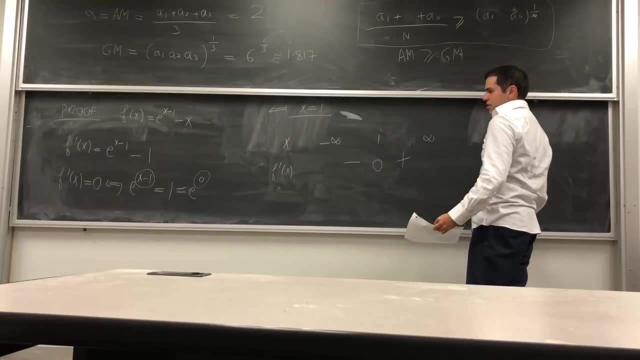 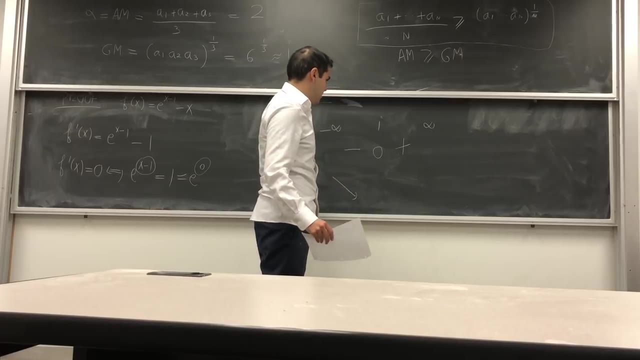 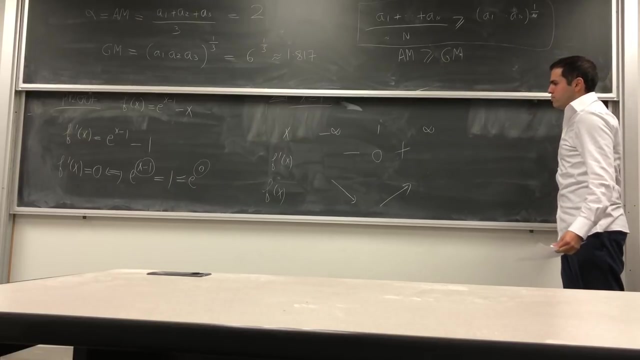 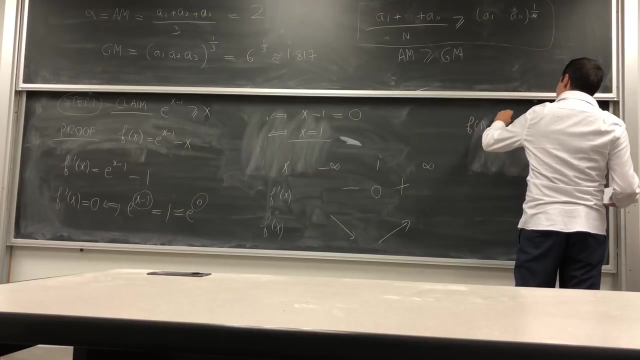 infinity to 1, the derivative is negative and on this interval the derivative is positive. So what does that tell us about our function? Well, again from calculus, it tells us that the function is decreasing here and increasing here. It still doesn't show that it's non-negative. but luckily, if you take f of 1, it's e to. 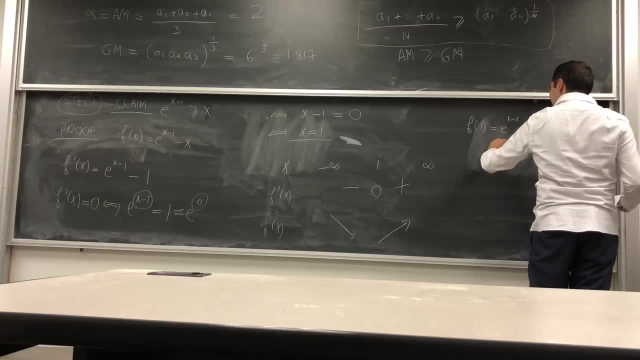 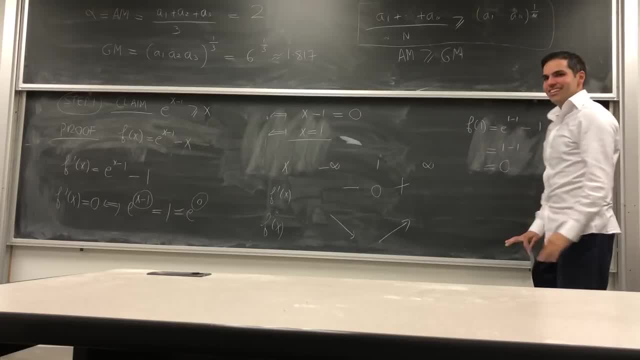 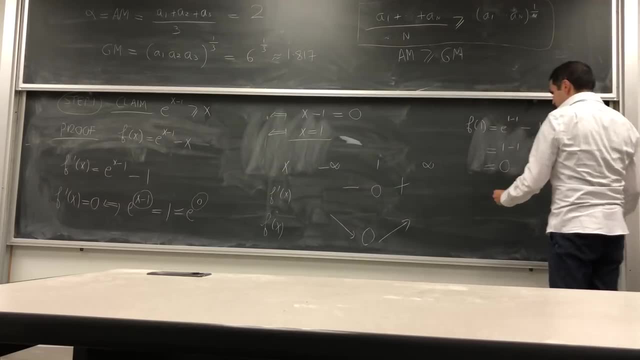 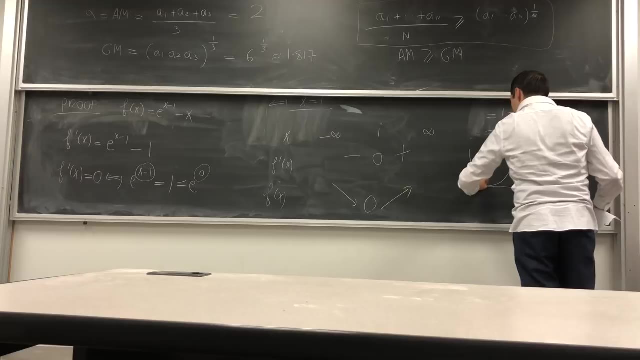 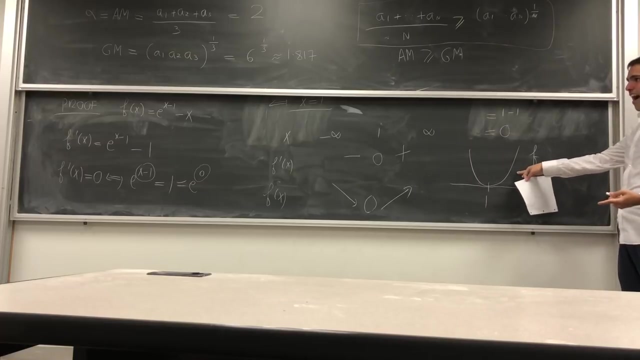 just 1.. OK, one is zero. so luckily in this case we find that F decreases to zero and then increases from zero on. so F looks something like that: at one it's zero, and then everywhere else is decreasing and then increasing. so in fact F of X is. 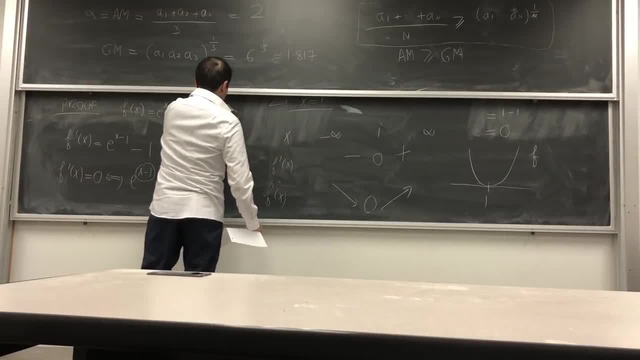 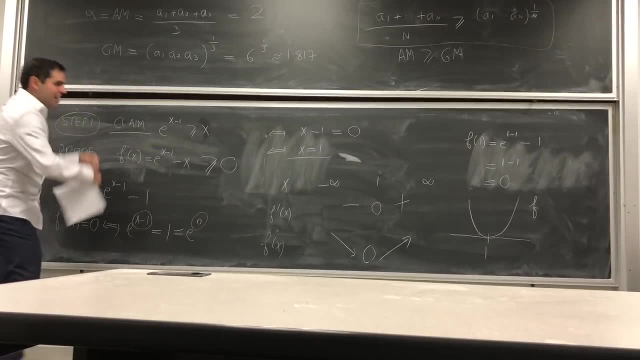 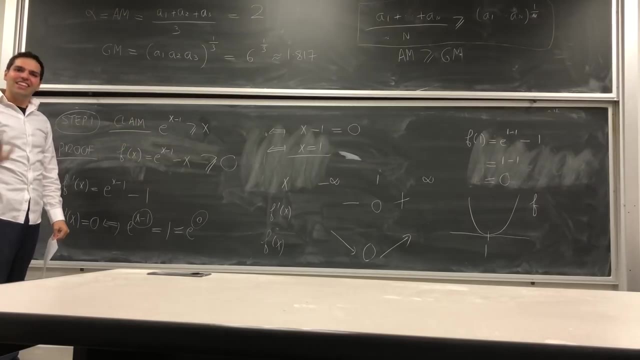 greater or equal to zero. this function is greater or equal to zero and therefore- and hit it, but let me unCON hide it- we get e to the X, minus 1 is greater or equal to X, so the calculus part of us is very satisfied, all right. second step: 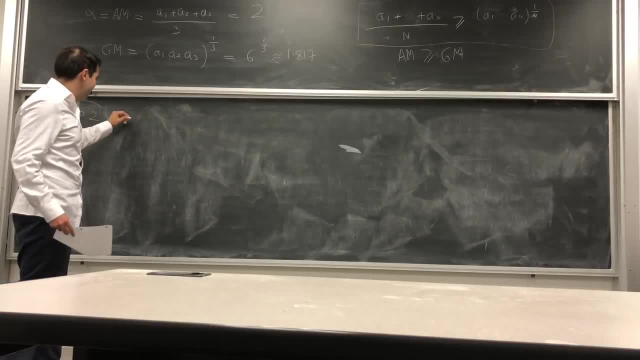 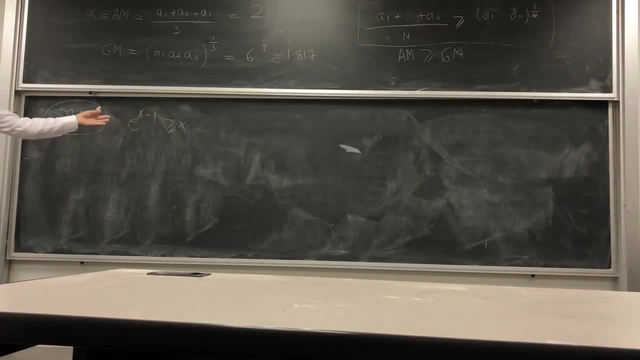 remember previously in my n battles called Galactica, we've shown that you- you take 1 is greater or equal to 0, so F is greater or equal to 0, and therefore I'm one is greater or equal to X. but now, how can we use this? well, of course you want. 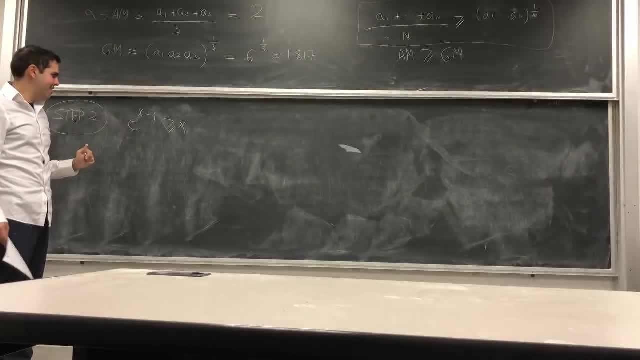 to figure out. you know, plug in the terms of our arithmetic, geometric mean, inequality. but just one little intuition. the nice thing is e to the X. it converts sums into products. and that's why we chose e to the X, because somehow it gives us a connection between products, so you know, or in between sums. so 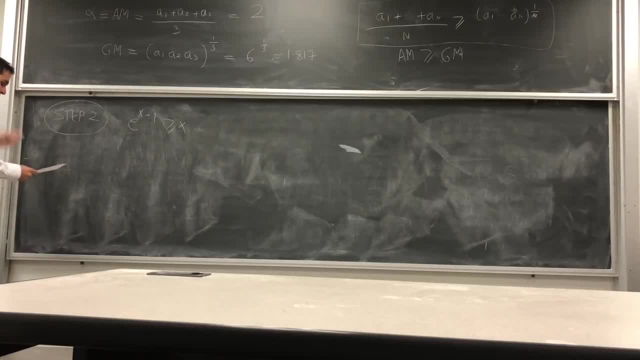 arithmetic stuff and products geometric stuff. so this motivates us to say that I let x equals to ai over alpha for each ion. well, I would like to remind you that alpha is just the arithmetic mean. A times A is the K related to A and delta is 32.. 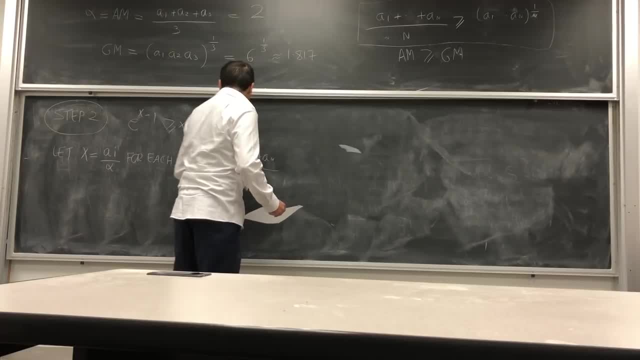 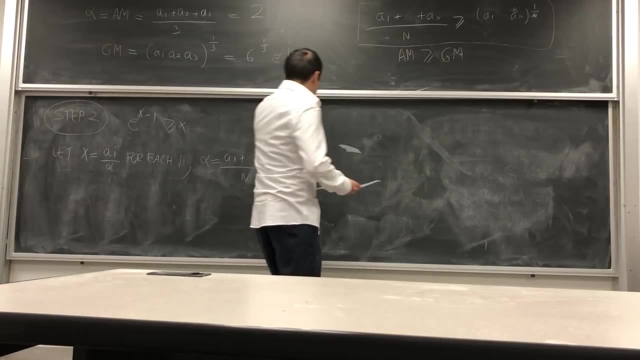 A times A is k, alpha is just the arithmetic mean right. and if we look at an example, let's say here A times i, elements on K symbols have some equals, and then what happens is that plus dot, dot, dot, plus a n over n. So what do we get here? We have that, first of all, e to 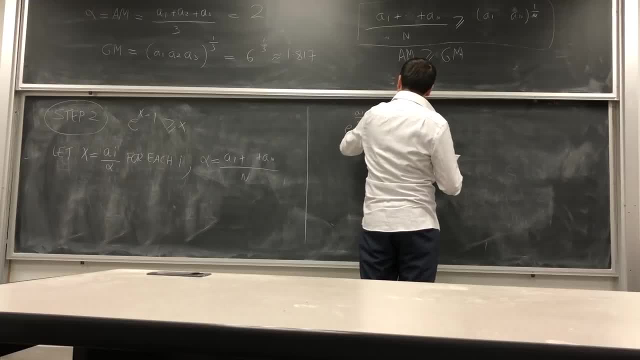 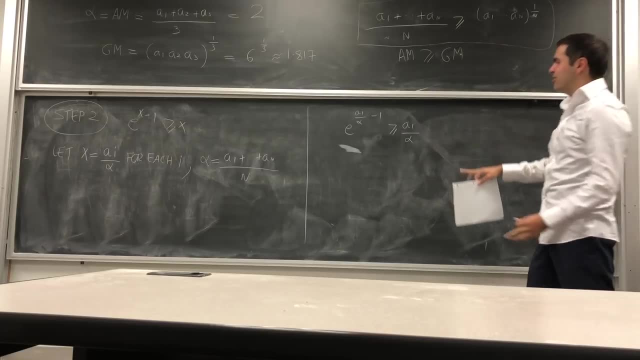 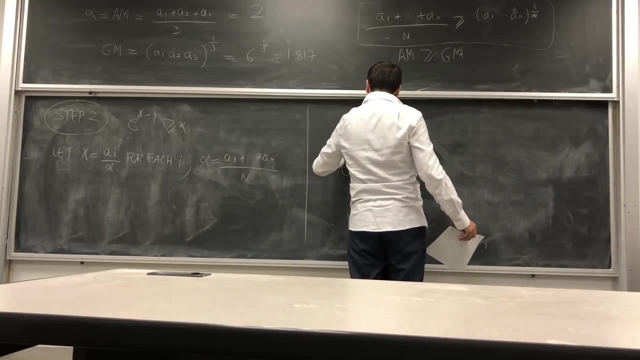 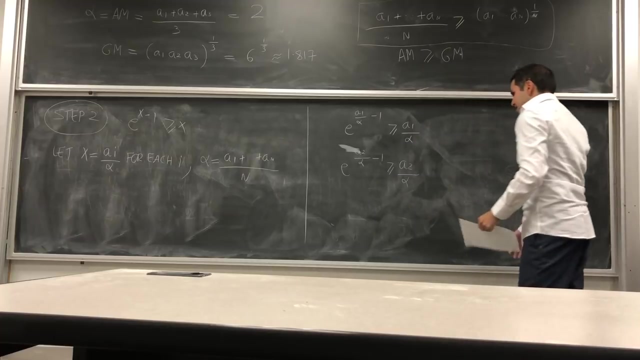 the alpha 1. a 1 over alpha minus 1 is greater or equal to a 1 over alpha. That's just by plugging in. x equals to a 1 over alpha. Now let's do the same spiel and do without a 2.. a 2 over alpha minus 1 is greater or equal to a 2 over alpha. and then 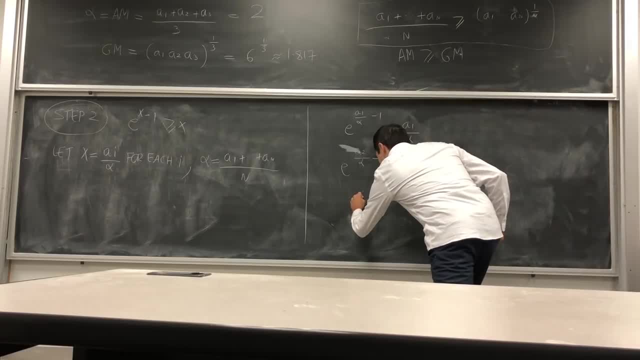 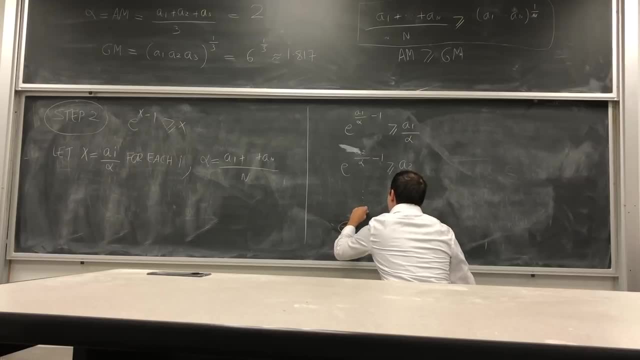 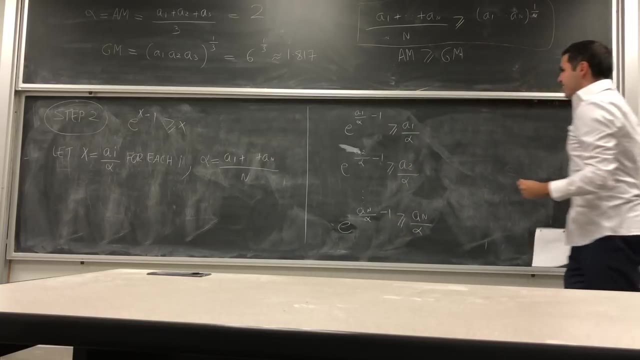 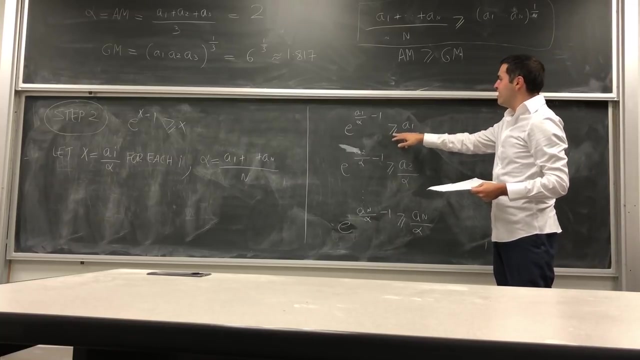 you can do the same thing and you get that e to the a, n over alpha minus 1 is greater or equal to a n over alpha. Great, By the way. you know just a little thing. when is this? when do we have an? 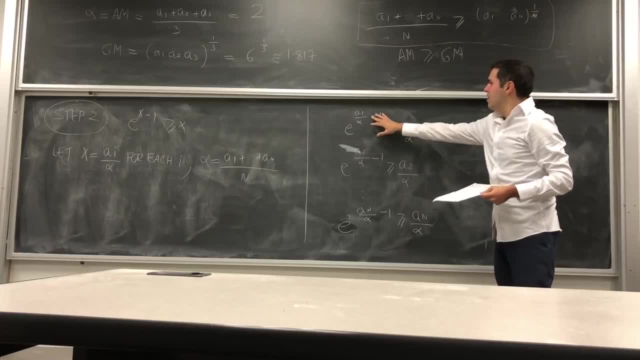 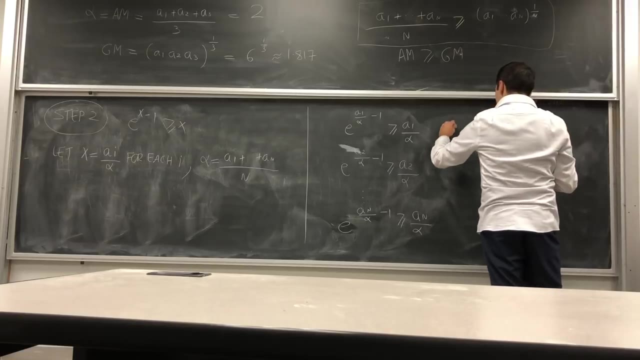 equality here, it's precisely when this thing is equal to that. and it's precisely remember. this function is zero if, and only if, x equals to one, and that's the case if, and only if, this thing equals to that. So not equality when a 1 over alpha is greater or equal to a n over alpha. 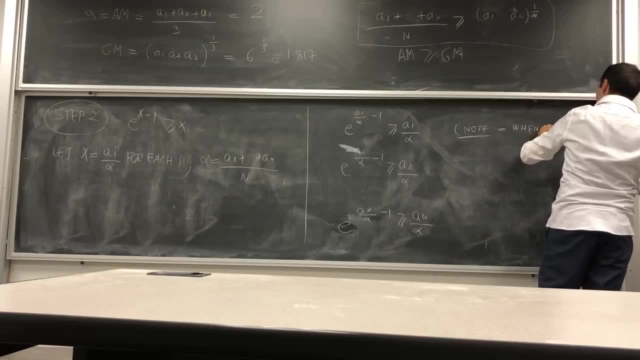 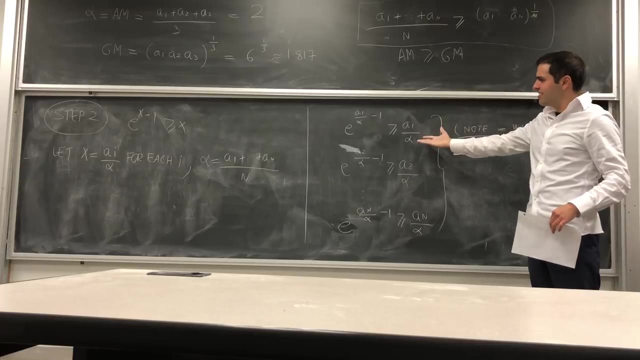 So no equality. when a 1 over alpha is greater or equal to a n over alpha, alpha equals to 1, and I'll talk about that in a second. But what do we have? We have a bunch of inequalities. and then the next thing to do: 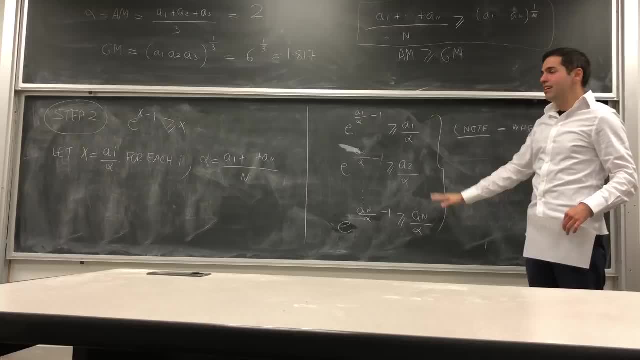 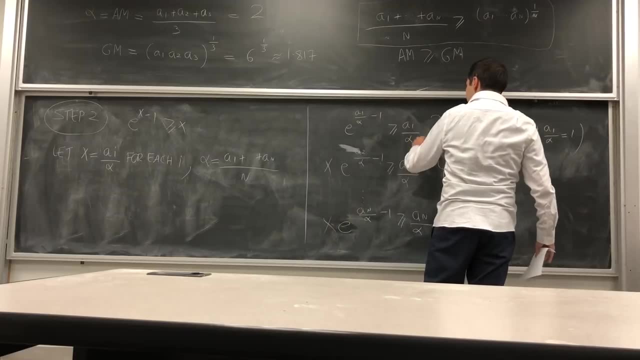 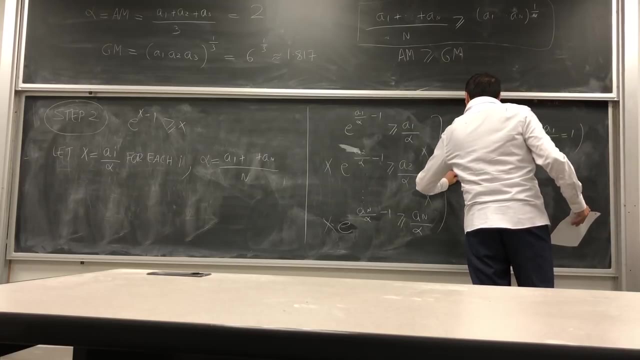 because ideally we would like to have a product of things is simply to multiply those things out. So you do this times, this times, this is greater or equal to this times, this times, this times, this, and then, if you do all this thing, you have e to the alpha 1 minus 1 over. sorry, 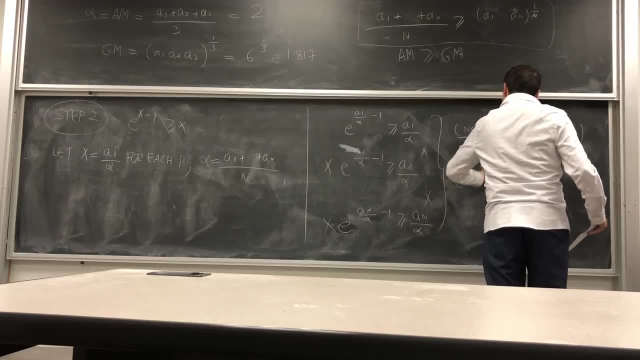 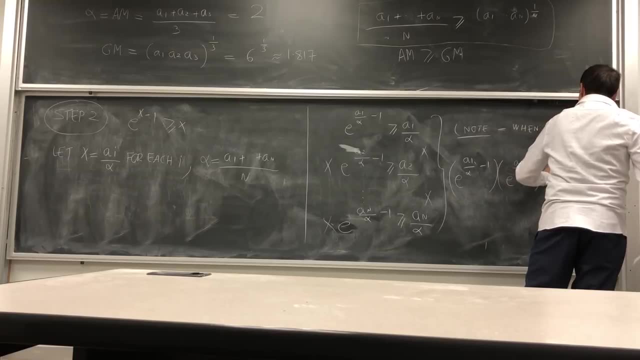 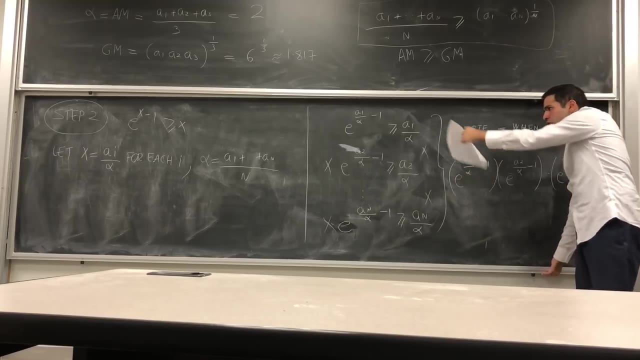 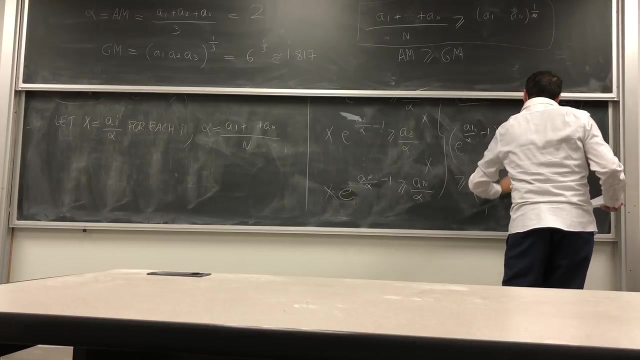 e to the a1 over alpha minus 1 times e to the a2 over alpha minus 1. dot, dot, dot. e to the an over alpha minus 1 is greater or equal to the product of all this junk. greater or equal to a1 over alpha, a2 over alpha, dot, dot dot. 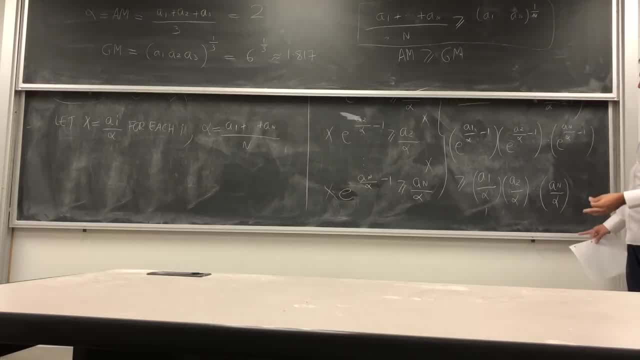 an over alpha. And, by the way, this is where we use the fact that all the ai's are positive. So we didn't multiply a positive number with a negative number, which would destroy our inequality. And second remark: now we have a product of everything. 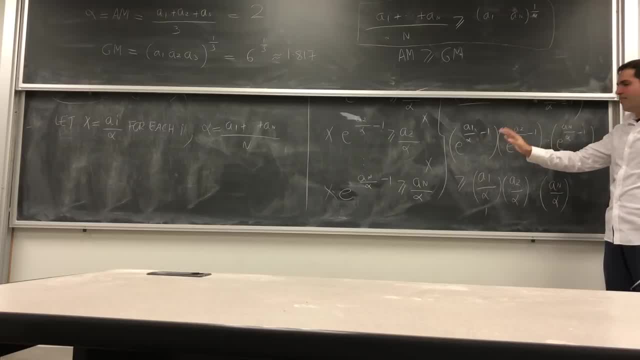 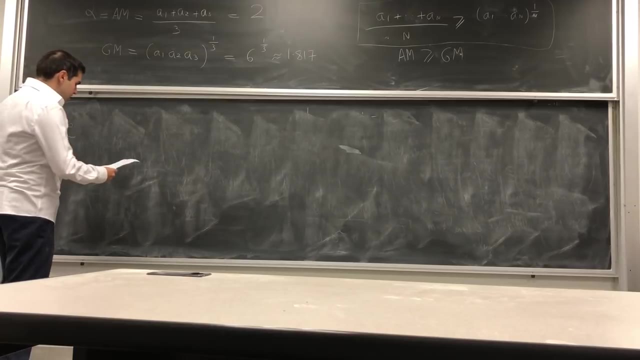 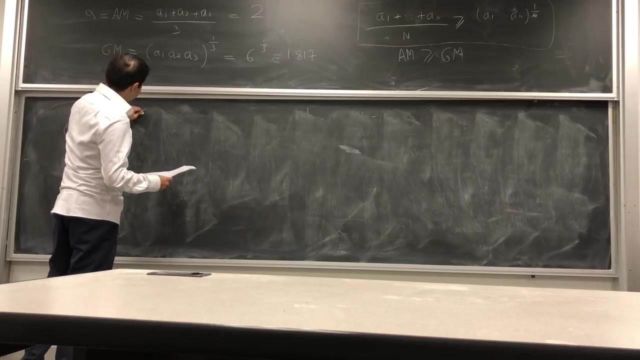 And remember e, e to the. something converts products into sums, And again we have this connection now between arithmetic means and geometric means. OK, so now, if we multiply everything out, we indeed get e to the a1 plus a2 plus dot, dot, dot plus an. 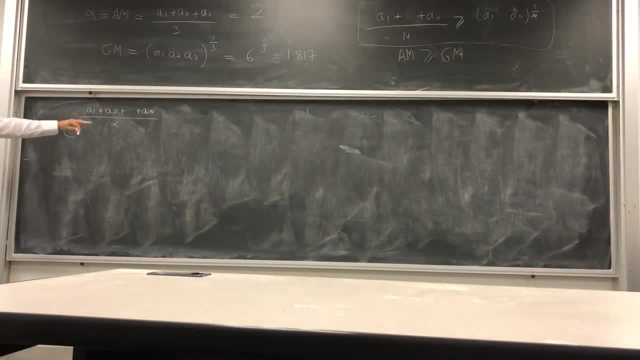 over alpha. So you just sum everything up And you have a common factor of 1 over alpha. And then the other thing is you sum up 1's, but how many times n times? So you get this thing: minus n is greater or equal to. again, 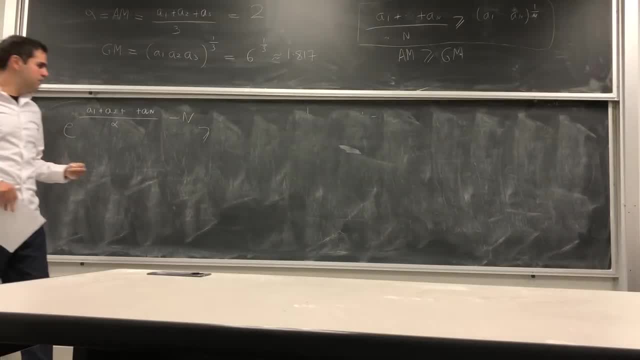 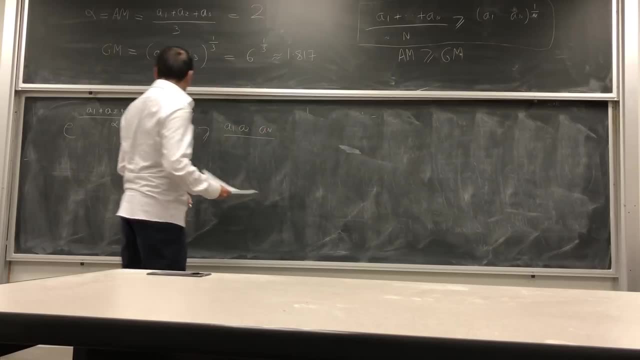 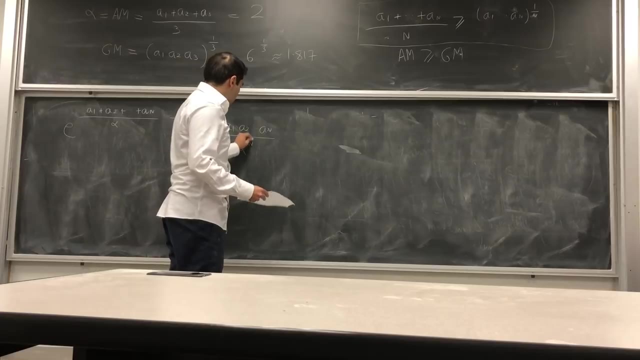 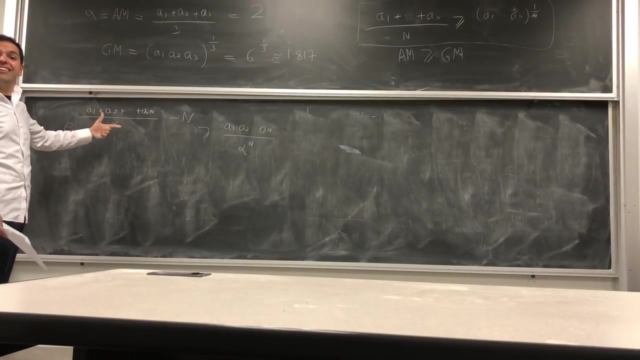 a1 over alpha times, a2 over alpha, et cetera, et cetera, which becomes a1, a2, dot, dot, dot, an over alpha. How many times? n times, because you're multiplying things n times. So alpha to the n, which is a better indication. 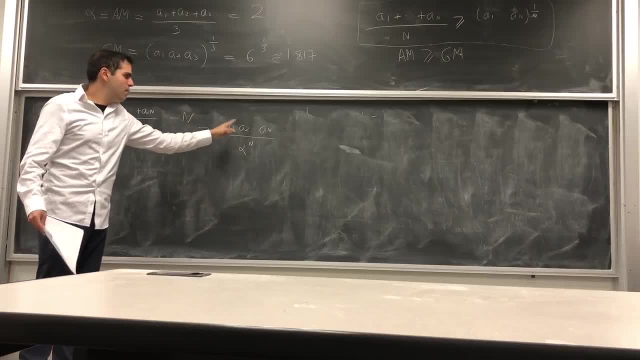 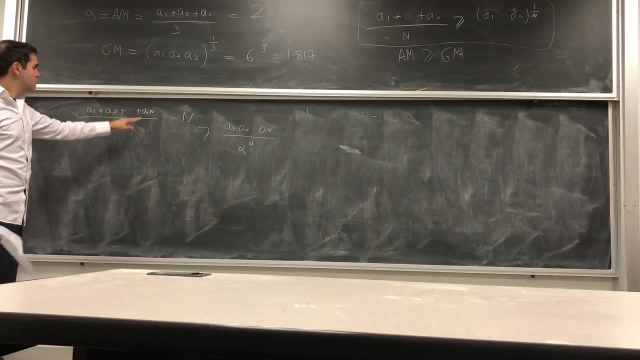 that you're right, because here we have sums of stuff, Here we have products of stuff, So we're closer to our arithmetic, geometric mean inequality. But it turns out this weird monster can be simplified OK OK. OK, OK, We like monsters, you know, but clean stuff up. 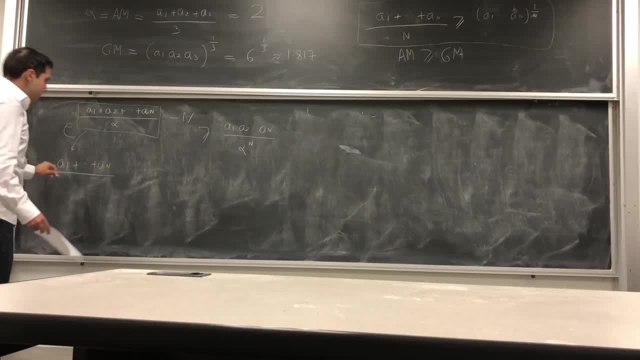 a1, this thing. what does that equal? to Remember that alpha is just the arithmetic mean. So it's a1 plus dot, dot dot plus an over n. And notice, you're in fact dividing this by this. So bang, bang. this cancels out. 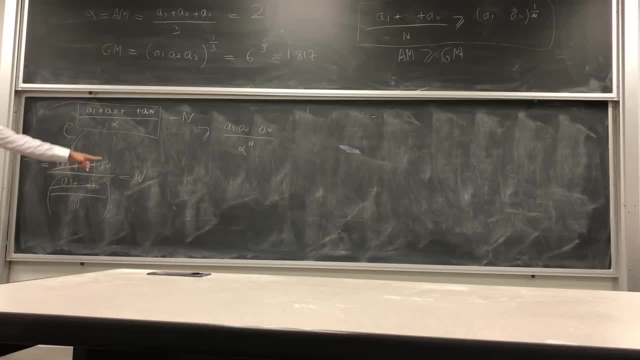 And, in the end, this weird monster, this monster equals to n, which is even better because this thing just equals to n And it in fact cancels out with this. So we have another- you know- explosion, And in the end, what you have is e to the 0. 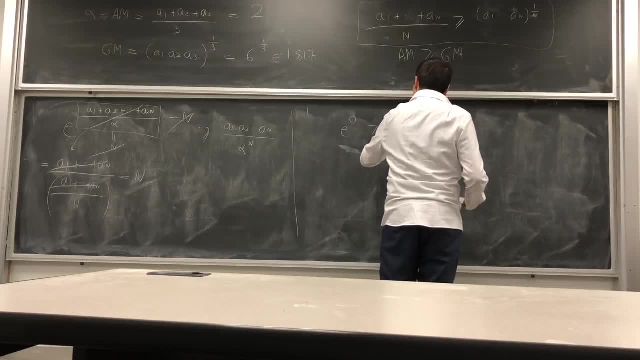 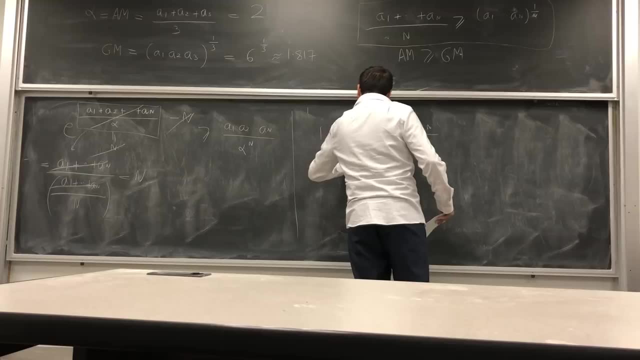 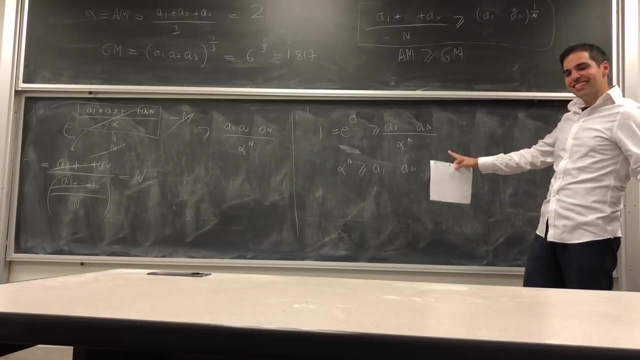 is greater or equal to a1. dot, dot, dot. an over alpha n e to the 0 is 1.. Cross multiply You get: alpha n is greater or equal to the product of an. And then, lastly, all you want to do is take the nth root. 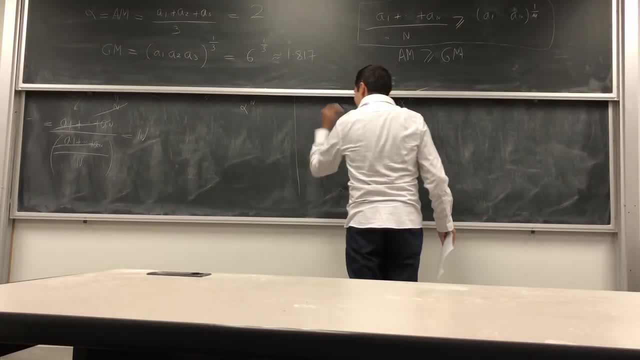 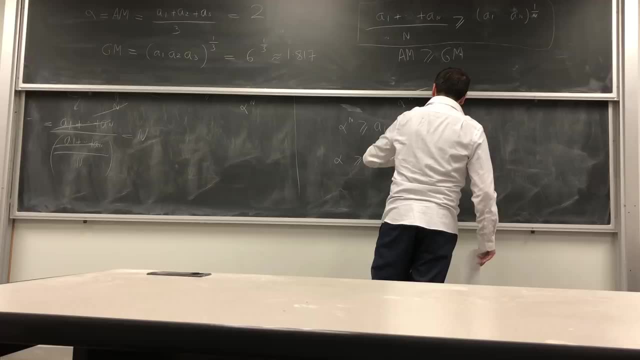 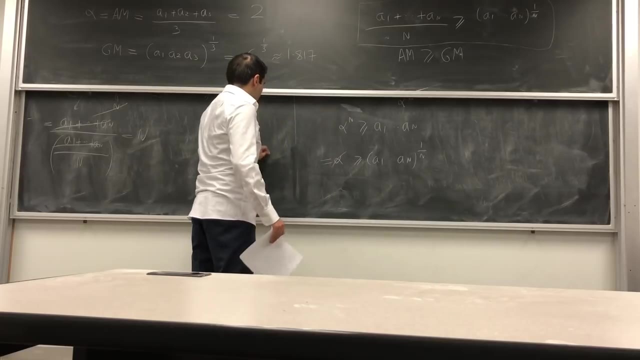 And again, everything is positive. So no worries about weird inequalities You get: alpha is greater or equal to a1, dot dot, dot, an nth root. But remember that alpha is just the same as a1 plus dot dot dot plus a n over n.